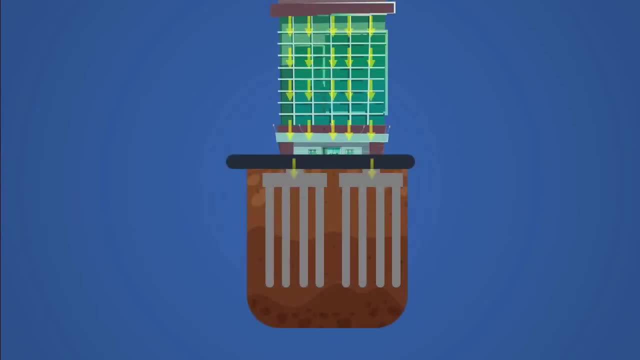 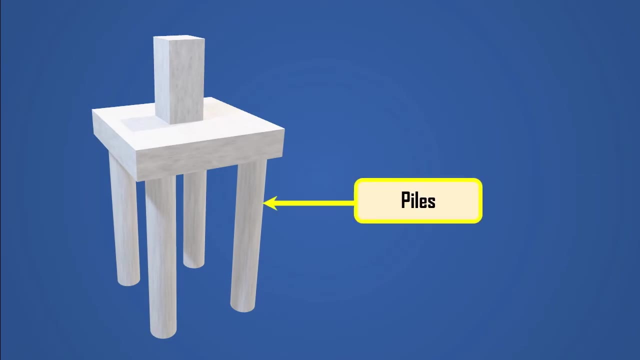 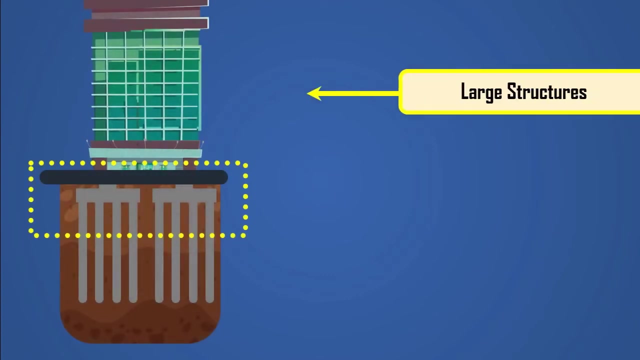 pile foundations. the loads are transferred to the hard strata through a vertical member known as piles. A pile is a slender member made of steel, concrete or wood. These types of foundations are usually used for large structures And in situations where the soil at shallow depth is not suitable to resist excessive. 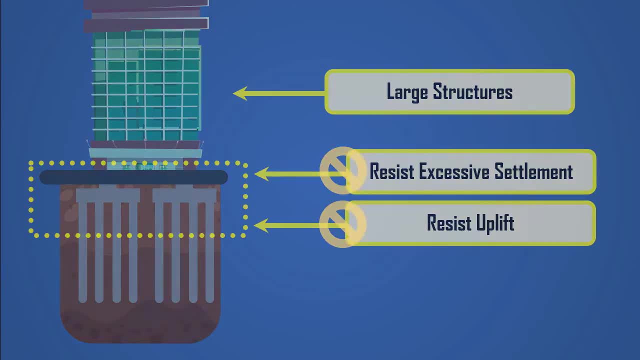 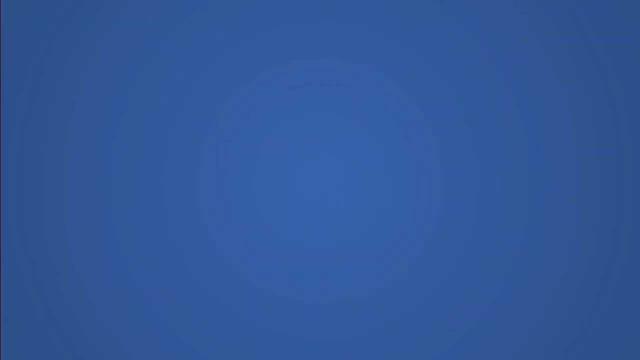 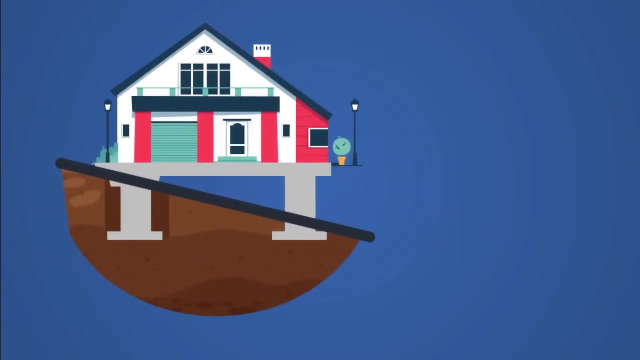 settlement, resist uplift, etc. Pile foundations transfer the load through both friction and bearing. Pile foundations can be classified based on function, materials and construction methods. We shall now move on to pier foundation. Pier foundation consists of cylindrical columns to support and transfer large superimposed 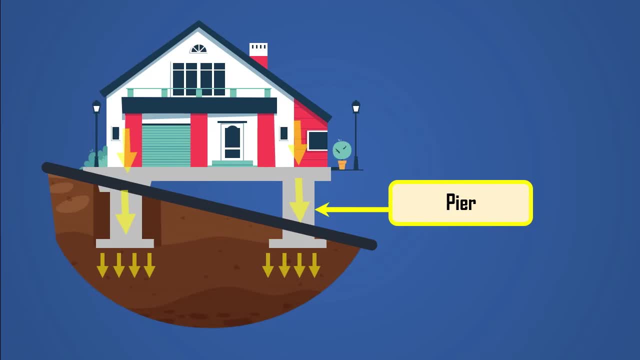 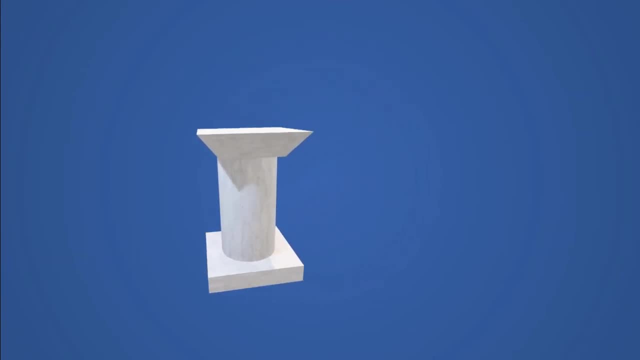 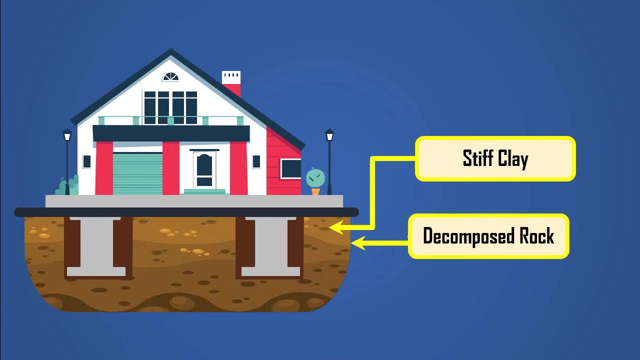 loads to firm strata. Pier is a vertical column similar to the pile but has a larger cross section. This type of foundation is used where top strata consist of decomposed rock, stiff clays, etc. Pier foundation is classified as a solid foundation. This type of foundation. 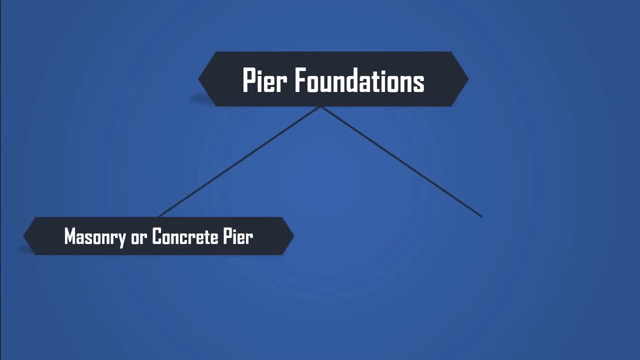 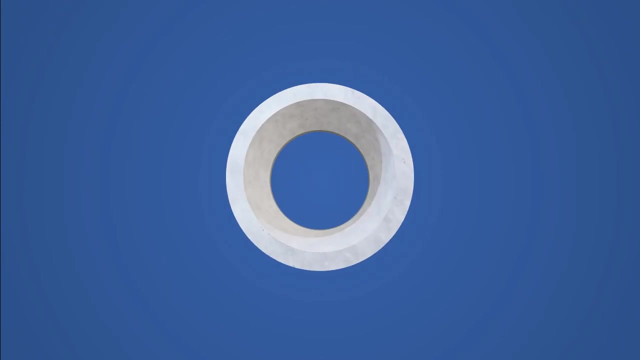 is used where top strata consist of decomposed rock, stiff clays, etc. Pier foundation is into two types: masonry or concrete pier and drilled caisson, Caisson or Well Foundations. A caisson is the type of foundation of the shape of a hollow prismatic box built above. 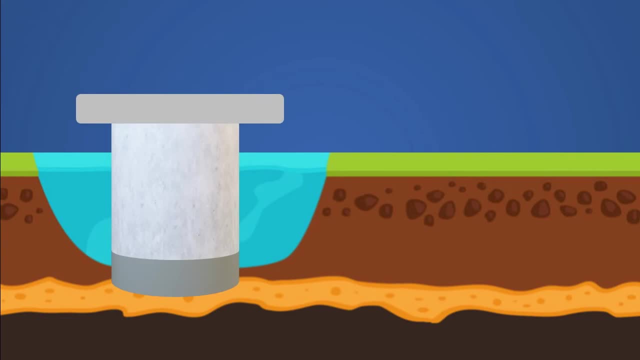 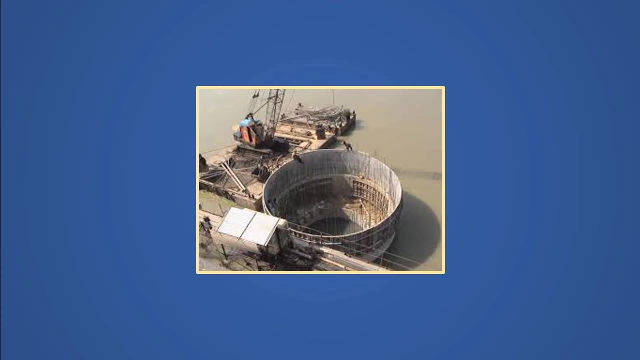 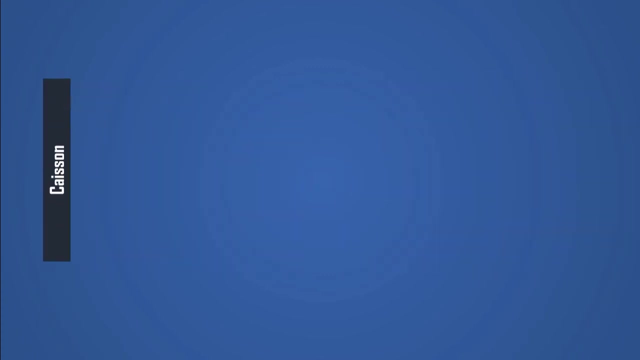 the ground level and then sunk to the required depth as a single unit. It is a watertight chamber used for laying foundation underwater, like rivers, lakes, harbors, etc. The caisson can be divided into the following three types: box caissons. 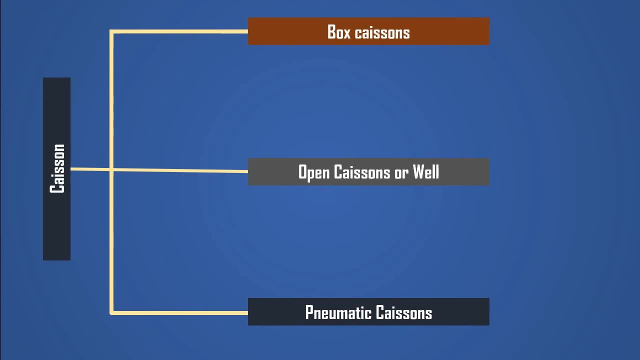 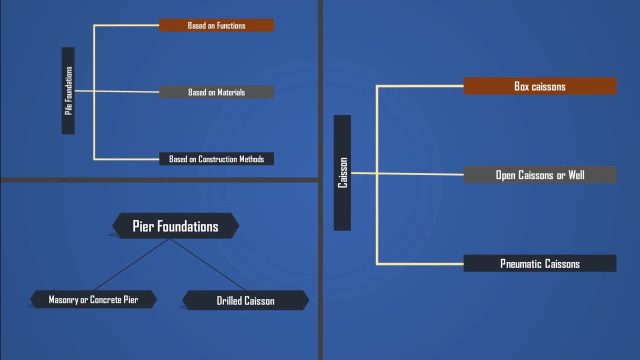 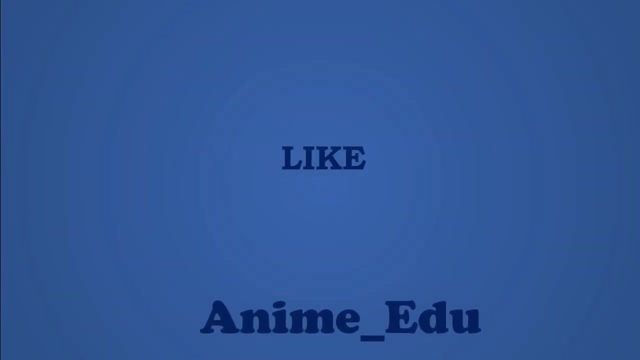 open caissons or well, and pneumatic caissons. We shall focus on each type of deep foundations in detail in upcoming topics. Thank you for watching. Stay tuned. The best is yet to come. Kindly do like, share, comment your views and finally, don't forget to subscribe to our channel.